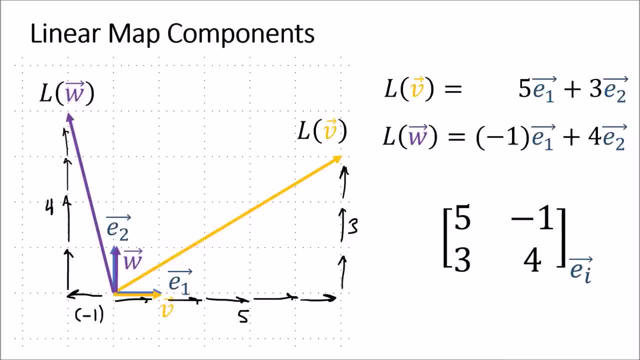 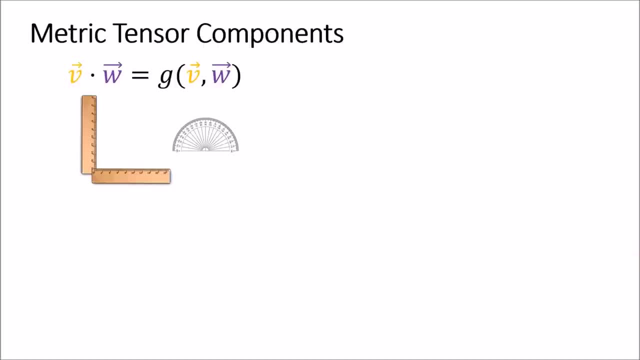 And usually we store the components of a linear map inside a matrix like this And, again, using different basis vectors, we would get different linear map components. And finally, metric tensor components are obtained by taking the dot products of all the basis vectors with one another and storing the results in a matrix And, as you probably know, the dot product 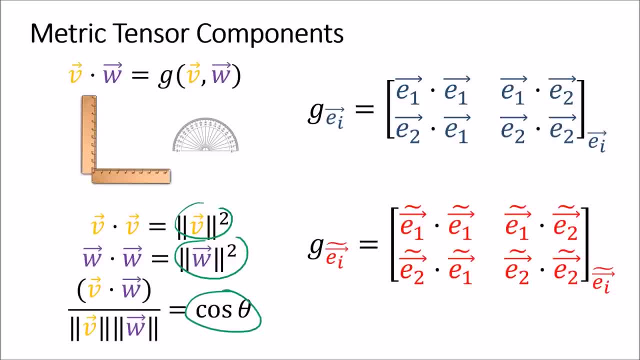 can help us get various matrix components. So let's take a look at the matrix components. So let's look at the matrix components From this. the matrix is a set of fixed vectors of different sets of weights and also able to combine the measures for various sets of vectors. 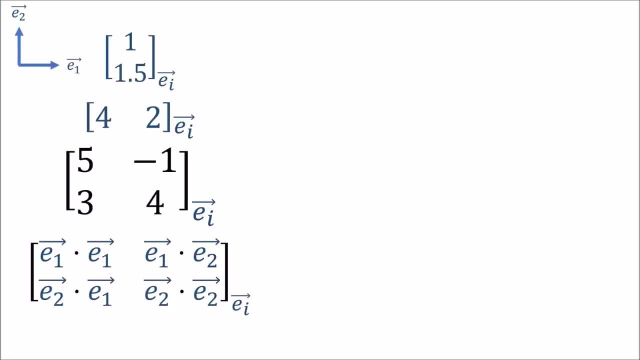 And then from that we can find the number of vectors and the set of vectors, as well as the angle that exists between a pair of vectors. So we know that when we have a tensor and a set of basis vectors, we can always find a way to measure the tensor's components using the set. 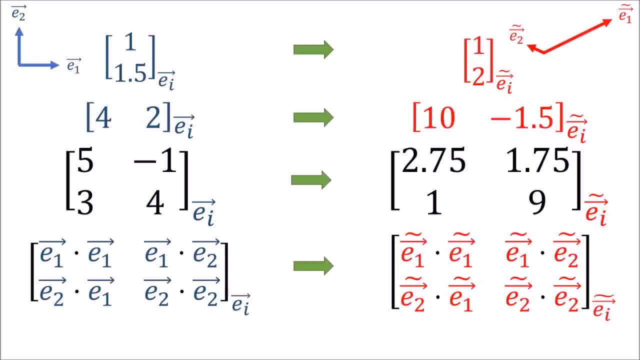 of basis vectors, And if we change the basis vectors that we're using, we're going to get a different set of components for that same tensor. So since the same tensor can have different components based on which coordinate system we use, we're left with the problem of how to convert. 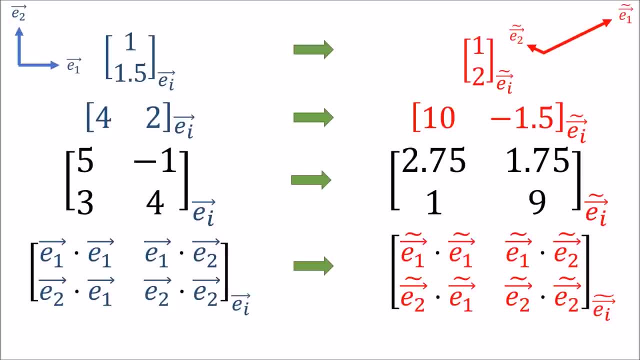 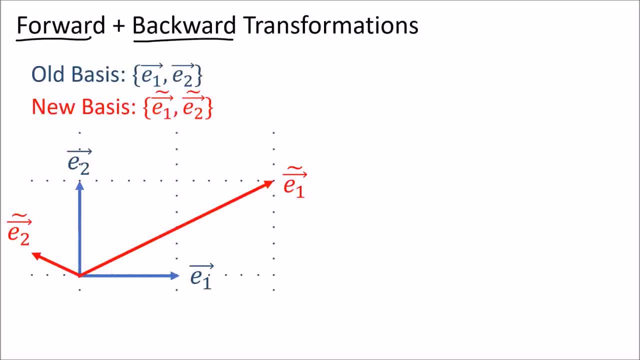 tensor components from one basis to another. And the secret to solving this problem is the forward and backward transforms When we have an old basis and a new basis. the forward transform is just the set of coefficients that we use to build the new basis vectors out of the old basis vectors and we can store. 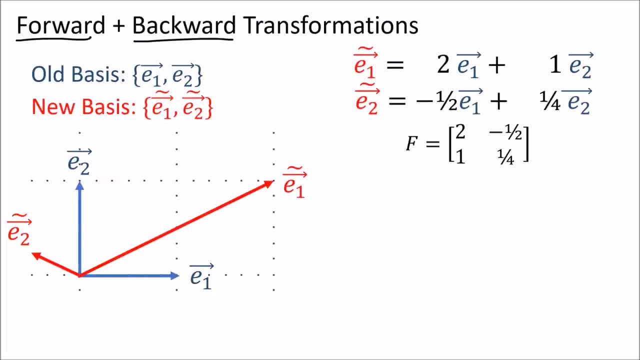 these coefficients inside a matrix called F. Likewise, the backward transform is just the set of coefficients that we use to build the old basis vectors out of the new basis vectors and we store these coefficients inside a matrix called B. B is the inverse matrix of F, which makes sense because the forward and backward transforms. 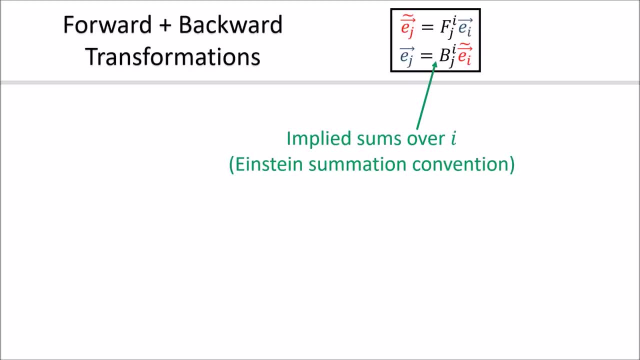 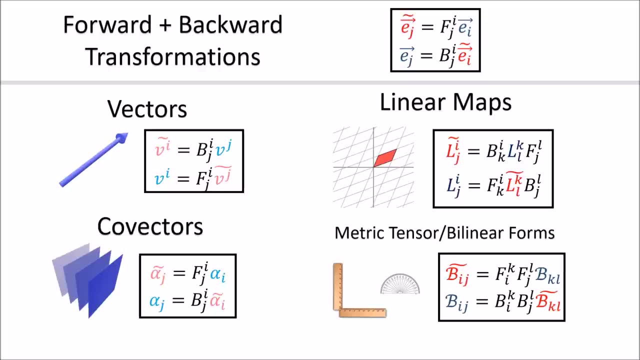 are opposite processes. So it turns out that if we know the forward and backward transforms for a pair of basis vector sets, then we automatically know how to transform the components of any tensor. We just apply some number of forward transforms and some number of backward transforms to 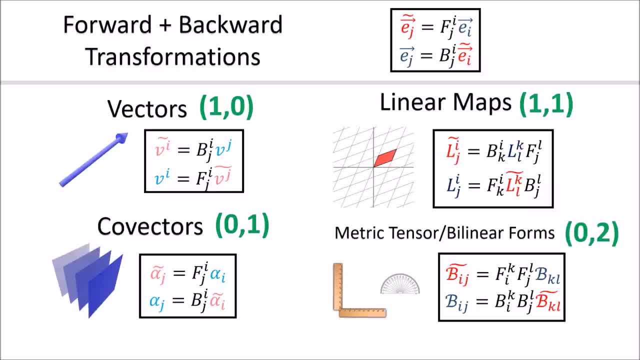 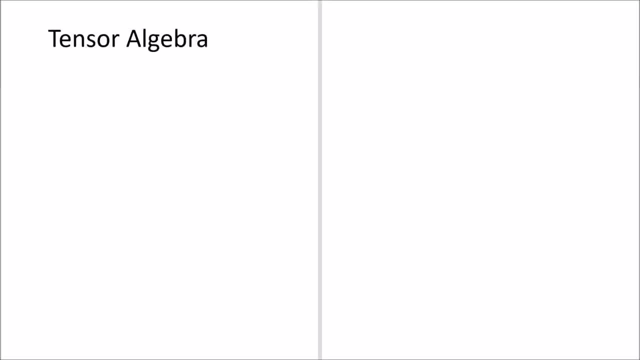 the tensor components, depending on the number of contravariant and covariant transformation rules that that tensor obeys. Okay, So all of that more or less sums up what you would have learned in my Tensors for Beginners video series, and all of this stuff is what I would call tensor algebra, which is the 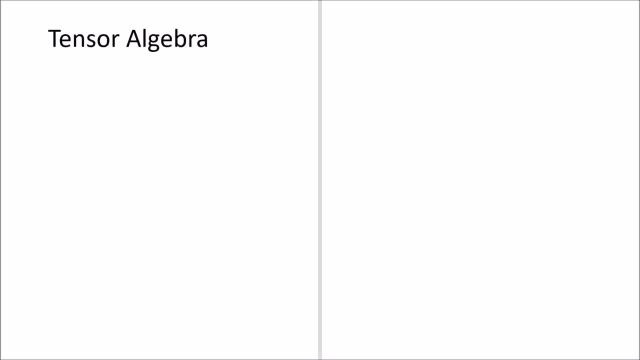 study of manipulating individual tensors in different coordinate systems. Now, in basic tensor algebra we usually consider only a few tensors at a time. We might take a pair of vectors, for example, and try to measure the angle between the vectors using the metric tensor. 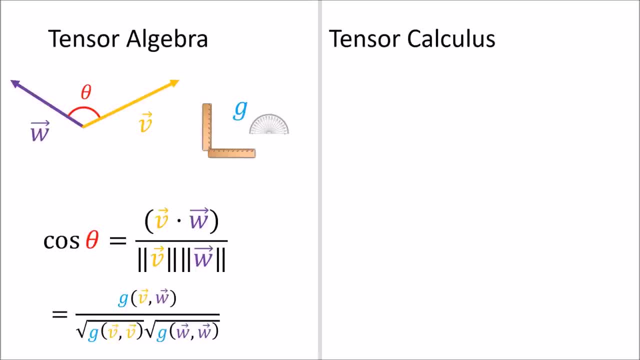 With tensor calculus, however, we stop dealing with individual tensors. Instead, we start considering tensor fields, which are infinite collections of tensors where the tensor changes at every point in space. If you studied multivariable calculus already, you're probably already familiar with the 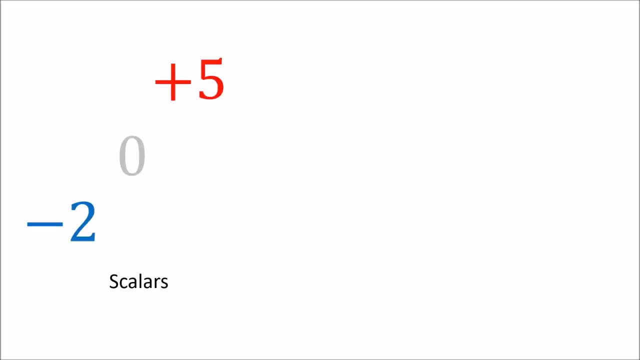 ideas of scalar fields and vector fields. Scalars are essentially ordinary numbers, but a scalar field is an infinite collection of numbers that varies everywhere over space. Temperature and voltage are examples of scalar fields from physics. You might also think of scalar fields as a number of vectors. 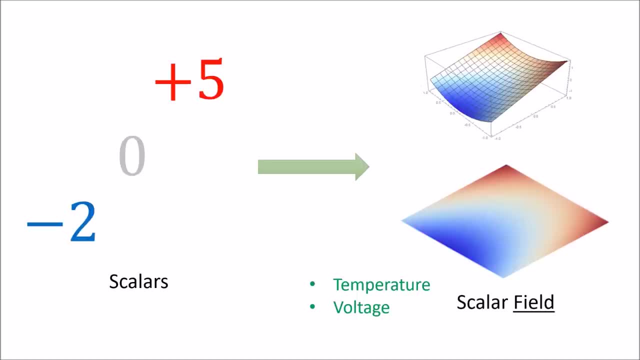 You might also think of scalar fields as a number of vectors. You might also think of scalar fields as a number of vectors. You might also think of scalar fields as just functions where the input is a point in space and the output is just a number. 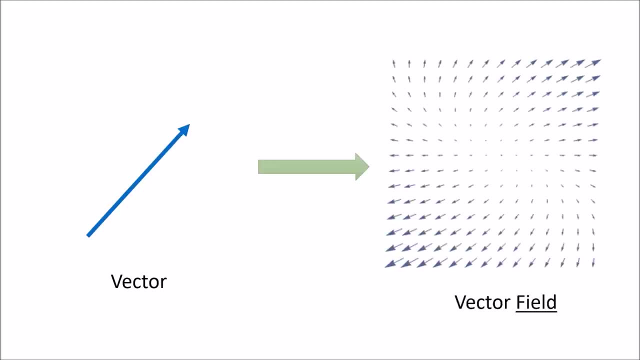 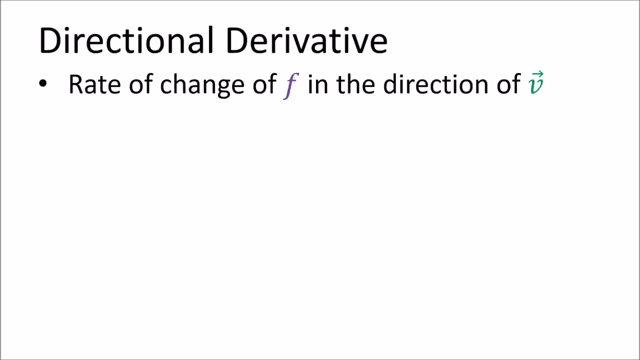 Also, rather than dealing with individual vectors, a vector field is an infinite collection of vectors where the vectors vary everywhere in space. The electric and gravitational fields are examples of vector fields that you would find in physics Using vector calculus. we can talk about how scalars and vectors change over space in 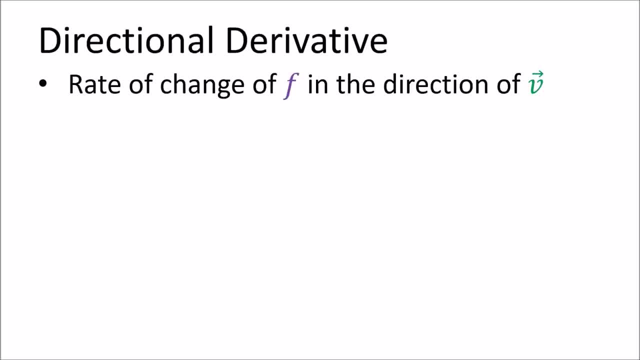 these scalar and vector fields. For example, we can consider the directional derivative of a scalar field. This tells us how the scalar field changes in a given direction. Tensor calculus is a generalization of vector calculus, where we consider not only scalar and vector fields but general tensor fields as well. 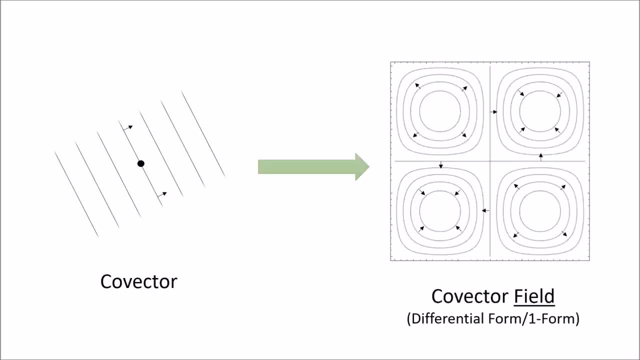 For example, instead of considering individual covector stacks, we consider covector fields, which are also called differential forms or one-forms, and these are fields where a different covector exists at every point in space. Also, instead of considering a single metric tensor that works as a vector, we can consider: 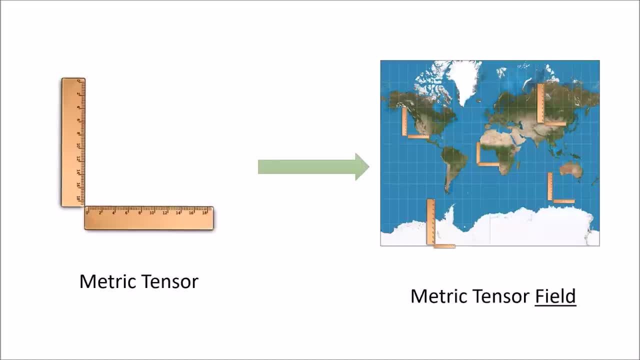 a metric tensor field where the metric tensor changes from point to point. A situation where this might come in useful is when we have a map of the Earth projected onto a flat plane. Because the Earth is a sphere, projecting it onto a flat plane will always lead to distortion. 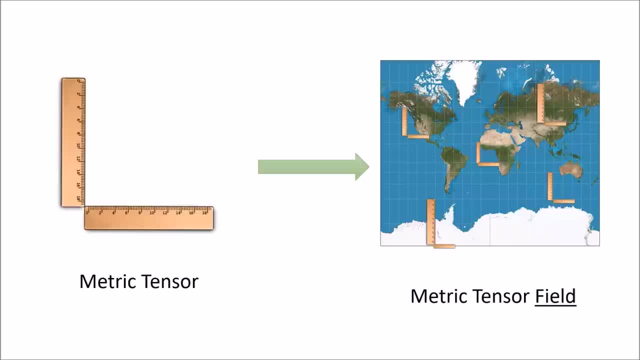 in the size of objects. So when measuring lengths and angles, we need to be sure to use the correct metric tensor for that region of space, so that we can measure sizes correctly. Also, in tensor calculus, instead of using a single vector field, we can use a vector. 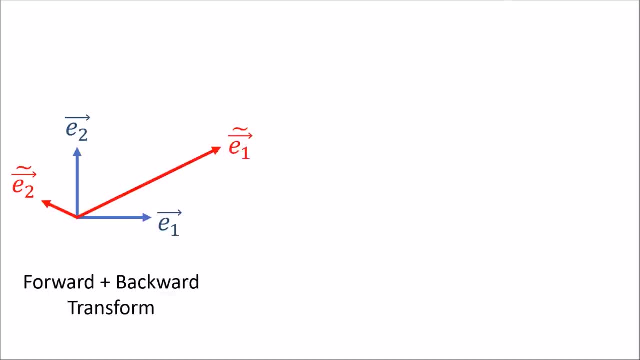 tensor. So instead of using individual coordinate basis vectors, we consider basis vector fields in a sense where the basis vectors will change from point to point everywhere in space. This is something you would find when changing from standard Cartesian coordinates to polar coordinates in 2D and instead of having a single forward and backward transform that 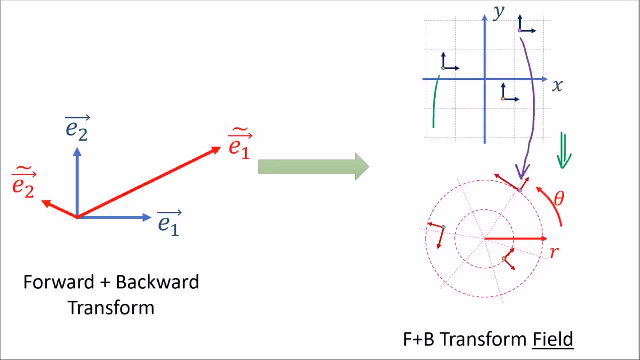 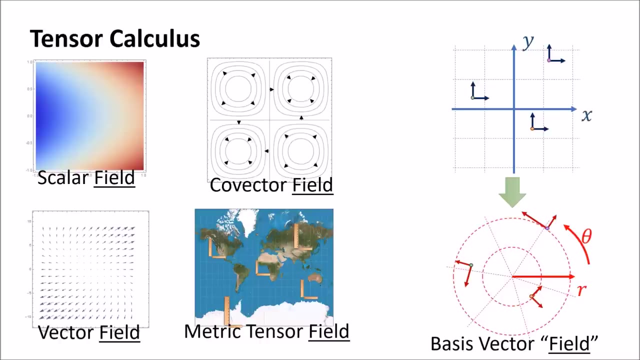 works everywhere in space. we have different forward and backward transforms for every single point, So it's almost as if we have a forward transform field and a backward transform field. So, to sum up, tensor calculus is basically the study of scalar fields, vector fields. 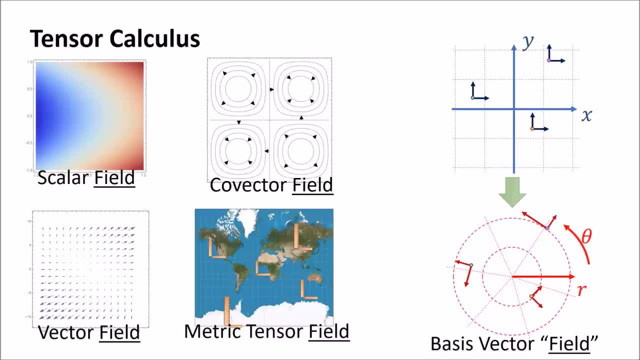 covector fields, metric tensor fields and any other tensor fields that we can come up with, And also how coordinate basis vectors change from point to point in space. So now that you know a bit about what tensor calculus is, why would you want to study it? 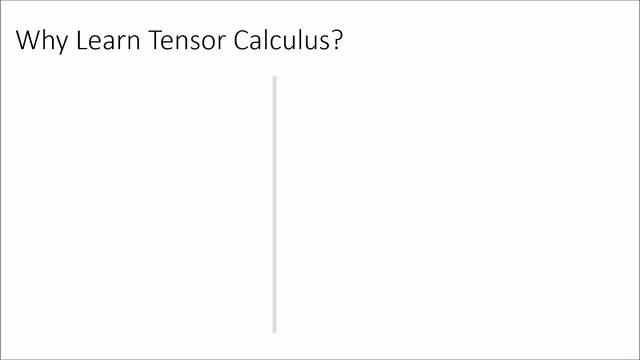 Well, it turns out that a lot of concepts in intermediate and advanced physics can be described by tensor fields. For example, you might be used to thinking of electric fields and magnetic fields as two different vector fields that are separate. However, we can combine electric and magnetic field vectors together into a single tensor. 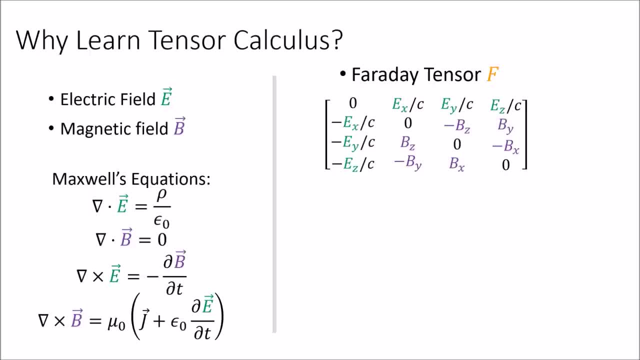 field given by the Faraday tensor, And the four equations of electricity and magnetism, which are Maxwell's equations, can be combined together and simplified into two tensor equations that describe the behavior of the Faraday tensor everywhere in space. This is usually how electricity and magnetism are described in special relativity. 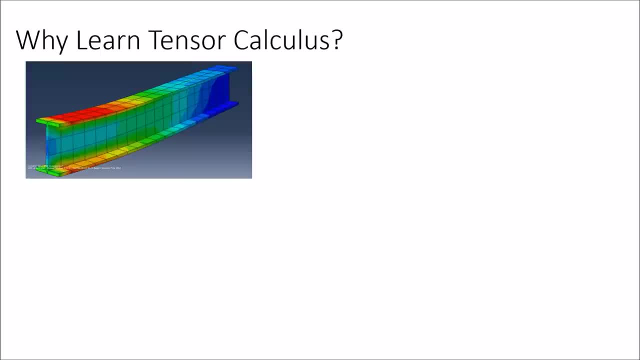 Another area where tensor fields are useful is in continuum mechanics, where we study the deformations of continuous materials under stress. The internal stresses and strains inside a material are given by the Cauchy stress tensor, which will vary from point to point inside the object forming a tensor field. 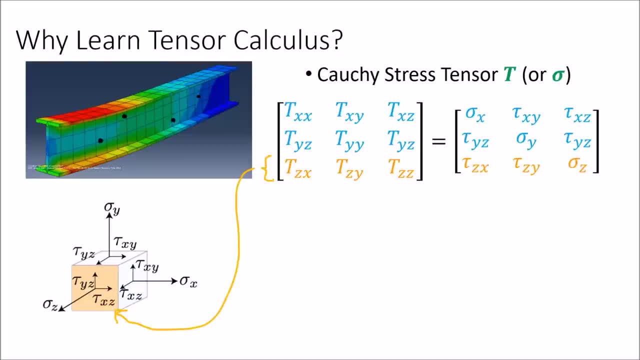 If we imagine all materials as being made up of small cubes, the T-I-J component of this tensor will measure the force vector on face I of the cube acting in direction J. This means that the diagonal elements of the tensor will measure normal stress, which. 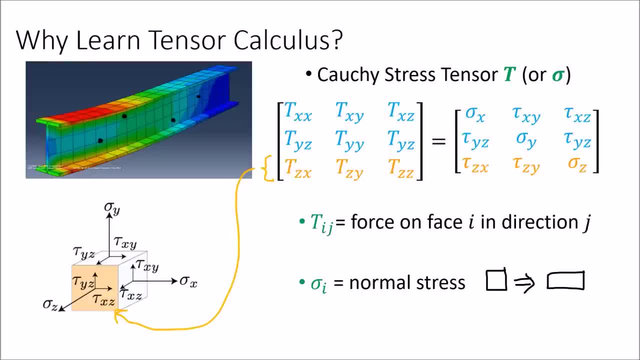 is basically like stretching and squashing of the cube, and the off-diagonal elements will measure shear stress, which are the stresses which are perpendicular to the faces of the cube. This can be used to study mechanical parts used in machinery, but it can also be used 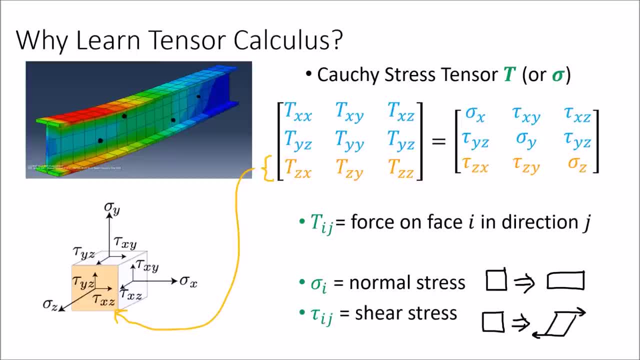 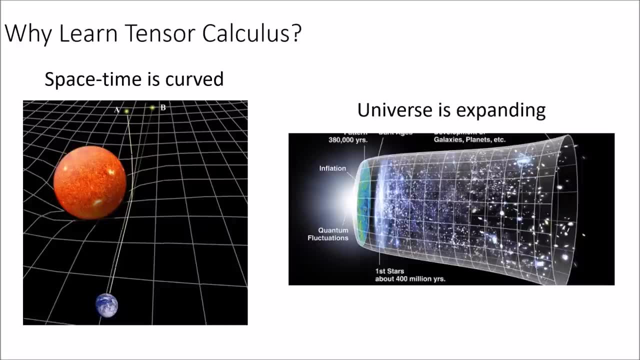 to understand the stresses of the Earth's tectonic plates which cause earthquakes. Thank you. A final example is in Einstein's general relativity, which is the theory that describes how energy and momentum can bend spacetime. This curvature of spacetime is the ultimate source of gravity in the universe and can. 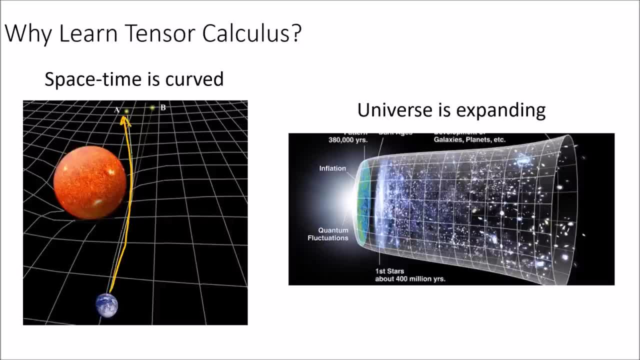 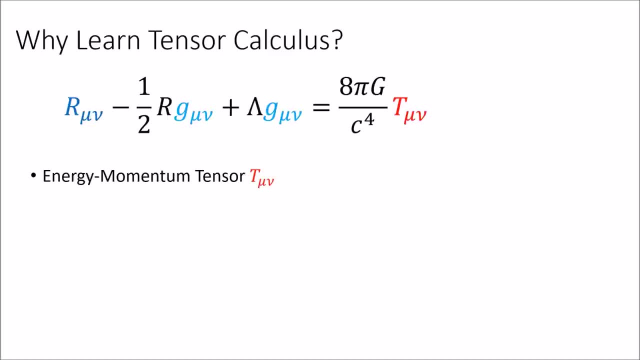 even cause light to bend from an apparently straight path if it's in the presence of enough mass-energy. It turns out that general relativity is full of tensors. There's the energy-momentum tensor, which describes how energy and momentum vary throughout spacetime. 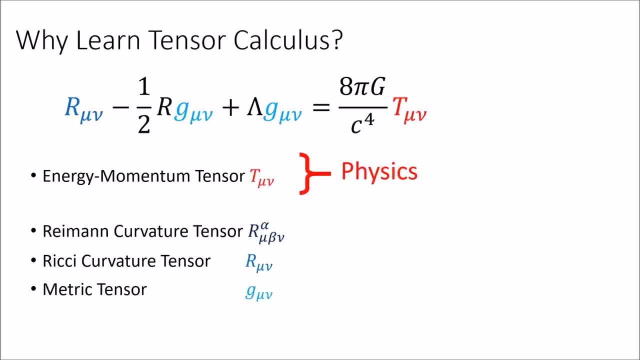 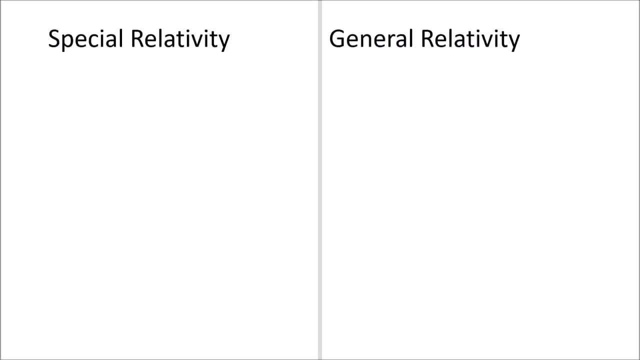 There's also the Ricci tensor, Riemann curvature tensor and metric tensor, which describe how spacetime curve and bend. In fact, one of the reasons why general relativity is so much more mathematically complicated than special relativity is because of the metric tensor. 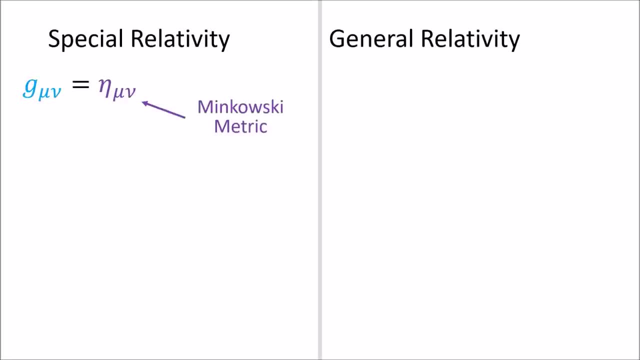 In special relativity there's a single metric tensor called the Minkowski metric, which is constant everywhere in the universe. In general relativity, the metric tensor will change at every point in space and time depending on how much energy and momentum is in the universe. 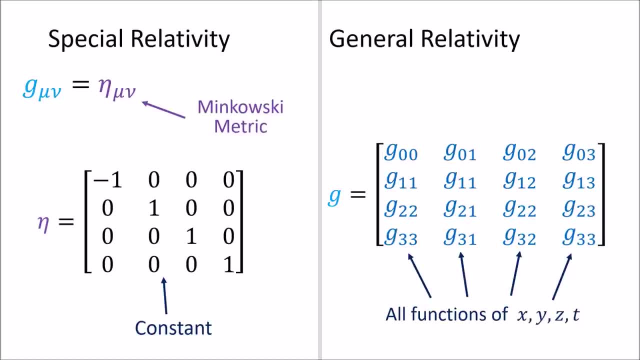 momentum is in the local region and since the metric tensor varies from point to point, we need tensor calculus in order to understand it properly. So all of that information might have been a little bit overwhelming, but hopefully it's given you some motivation to learn tensor calculus, even if you don't understand all. 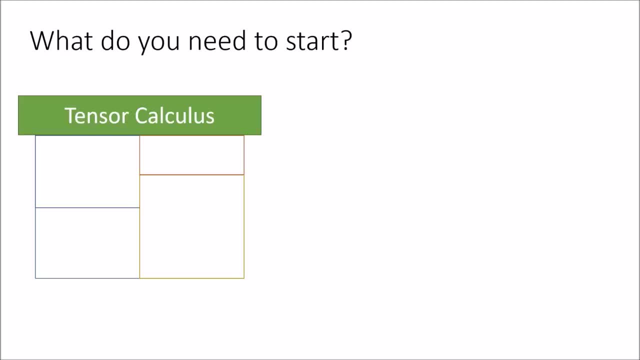 of that right now. So the final question is: what do you need to do in order to learn tensor calculus? Well, the rest of this video series is going to be dedicated to helping you learn tensor calculus, but I do have some advice before you start. 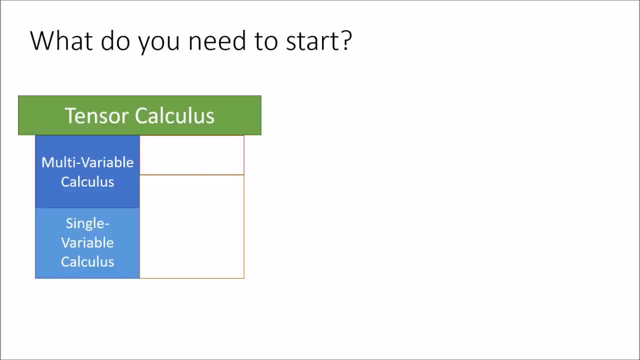 First of all, you need to be relatively comfortable with concepts from multivariable calculus. There's really no way getting around this, since tensor calculus is built on top of multivariable calculus. If concepts like partial derivative, gradient line, integral and directional derivative 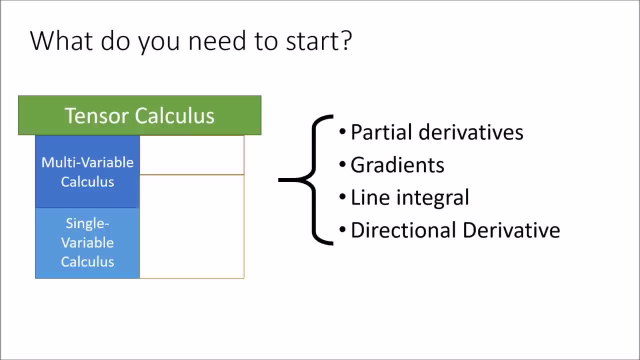 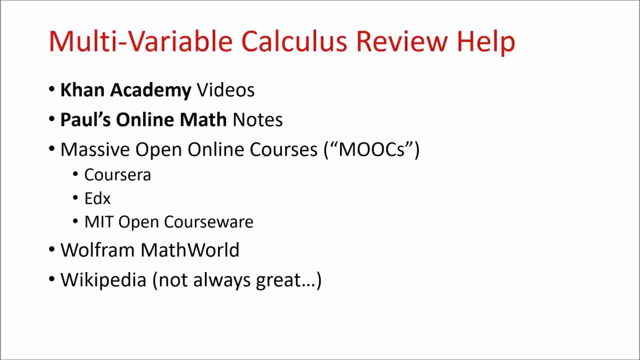 don't sound familiar to you. these videos might be a little too advanced for you right now. However, there are a lot of free resources online that can help you learn multivariable calculus. If you've already taken a multivariable calculus class, but you're a bit rusty, I'm going 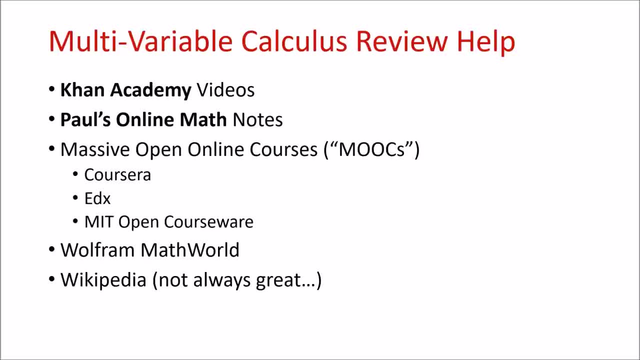 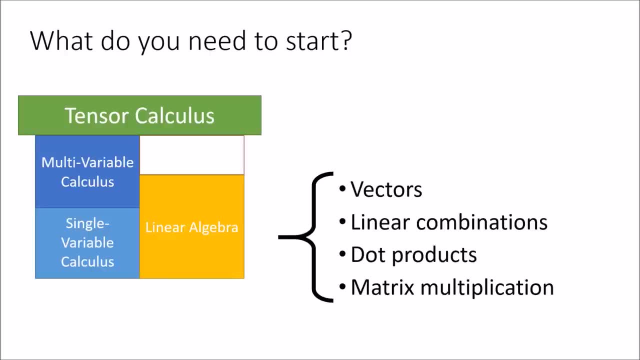 to do a very quick review of multivariable calculus in my next video to help refresh your memory. Next, it's important to be comfortable with basic concepts from linear algebra. You should understand concepts like vectors, linear combinations, dot products and matrix. 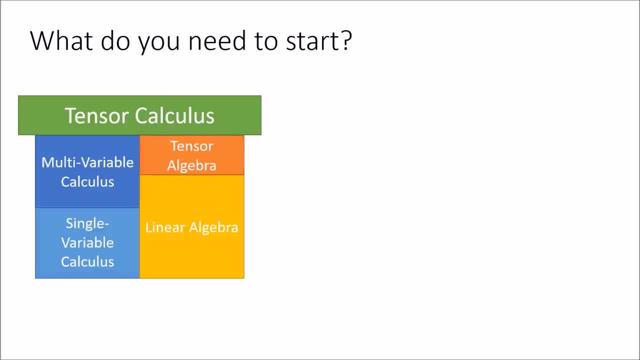 multiplication. Also, it's my personal opinion that before studying tensor calculus, you should also spend a little bit of time studying tensor algebra. This might make you a little worried, as a lot of people have never heard of tensor algebra before, but a lot of tensor calculus courses jump straight into tensor calculus. 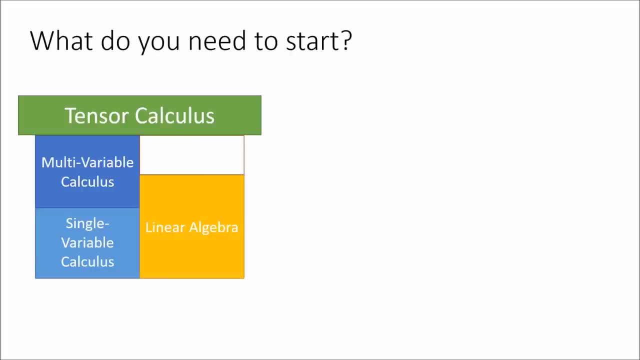 without covering tensor algebra at all. I personally feel like this is a mistake. To me, jumping straight into tensor calculus without doing tensor algebra feels like skipping a really important step, and you end up paying the price later on for not having a good foundation. 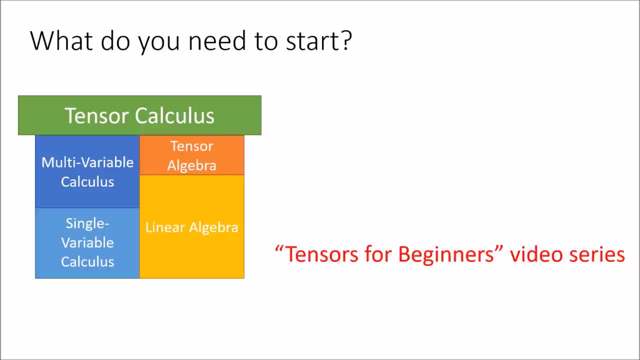 at the beginning. The good news is that I already have the video series called Tensors for Beginners that will teach you the basics of tensor algebra. The series is about 3 hours long, but I would say you only need to watch the first hour. 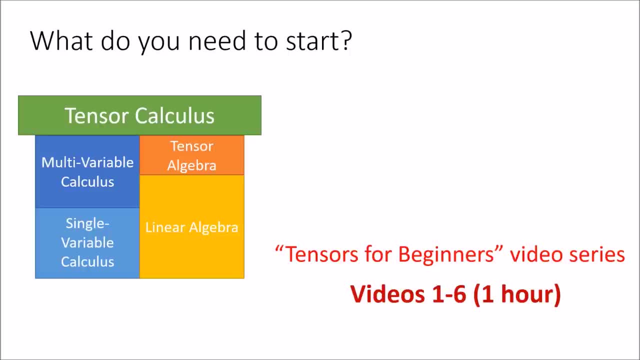 or so to get started. So before going forward with the tensor calculus videos, I would strongly recommend you watch videos 1 through 6 of my Tensors for Beginners series. This should get you familiar with forward and backward transforms between coordinate systems, as well as the ideas of vectors and covectors and how their components change. 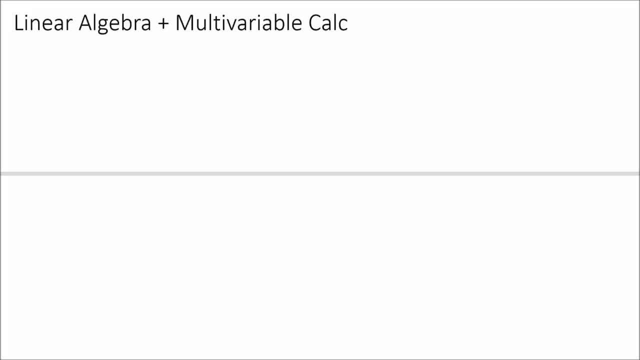 in different coordinate systems. The last piece of advice I'm going to give you is to warn you that when studying tensor calculus, we will often take mathematical symbols that you're familiar with and reinterpret the symbols to give them new meaning. For example, if you know multivariable calculus and linear algebra, you might see these symbols.